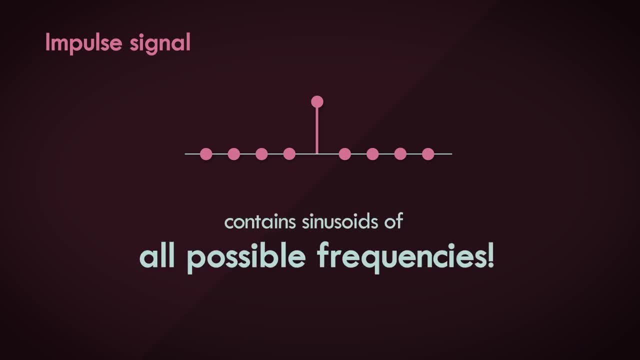 sinusoids of all possible frequencies representable for that sampling rate. This may be difficult to appreciate and certainly hard to grasp, But it practically contains all possible frequencies. Because of this property, the impulse signal is very useful in systems analysis and in 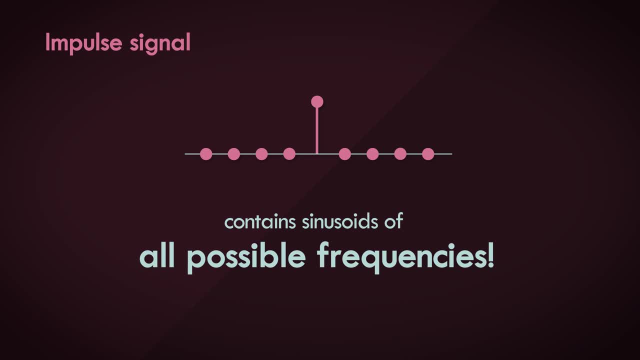 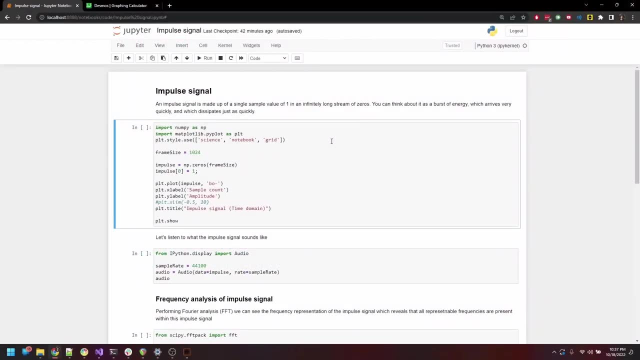 this particular series, filter analysis, as we'll soon see. But first let's actually create an impulse signal and put its wild claim to the test. I'm going to use Python to create a test signal and subject it to spectrum analysis. I'll 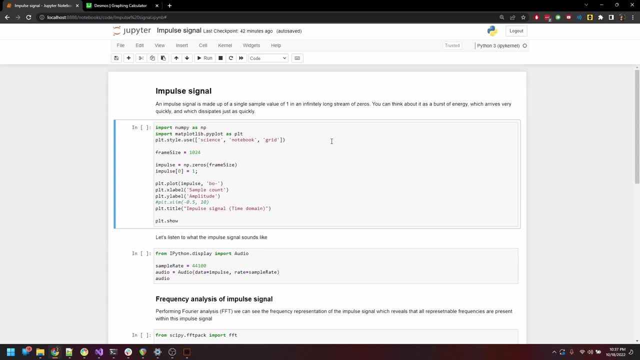 make the scripts available as Jupyter Notebook projects so that you may be able to interactively try these out in your own machines. if you're interested In another video, we can go through the scripts in more detail, but in this video I'll brush. 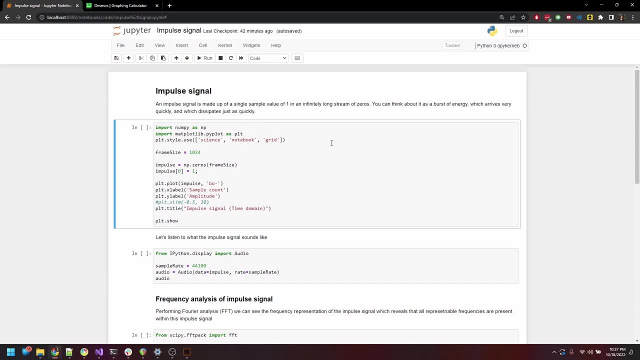 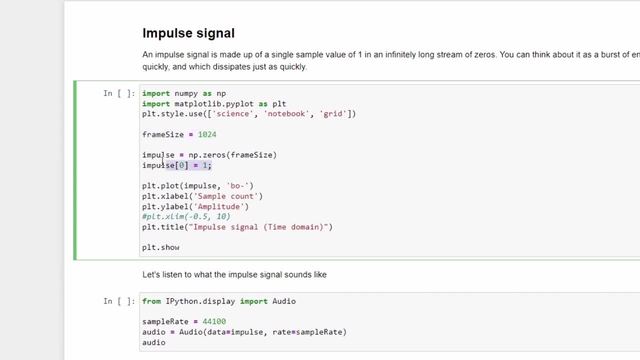 past the details and get cracking Here. I'll create a stream of zeros, say a length of 1024 samples. For the very first sample, I'll assign the value to be 1.. This is our impulse signal And if we plot it, 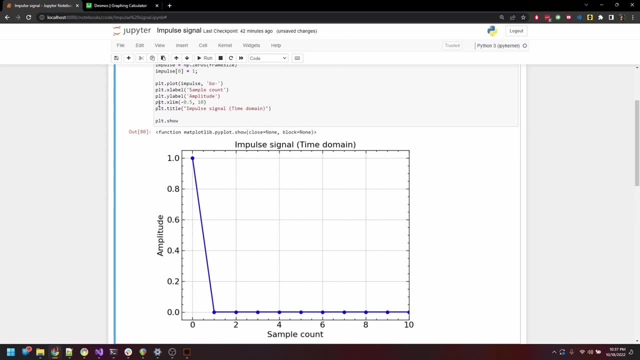 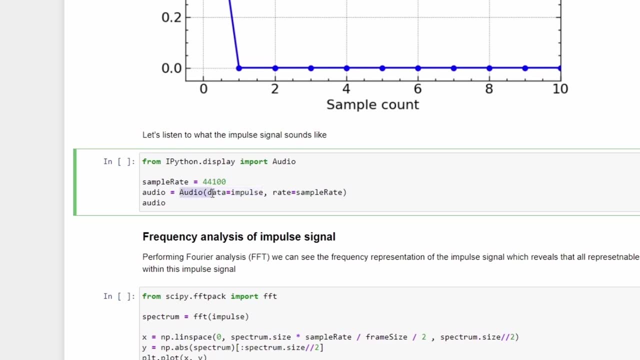 we can see the time domain graph of the impulse signal with a single peak. Here are what it sounds like as well. I'm going to take the stream of numbers and feed it into a function which will interpret it as sound and we'll set the sampling rate. 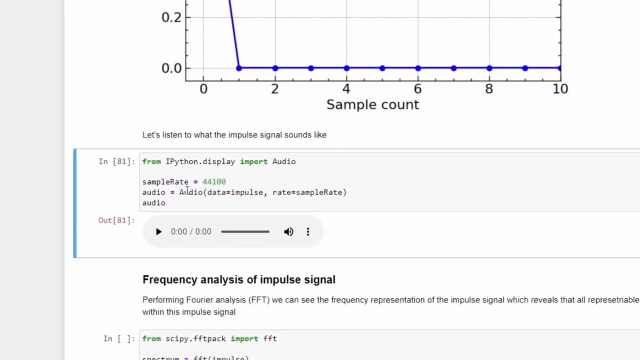 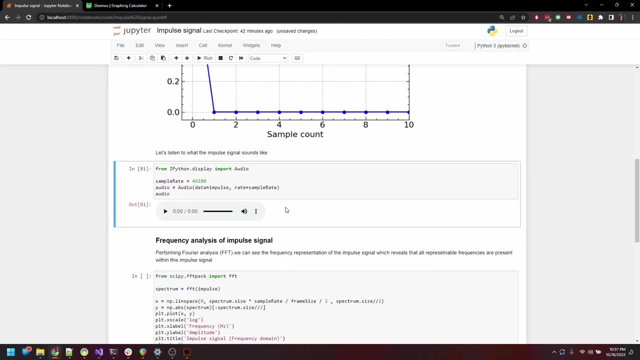 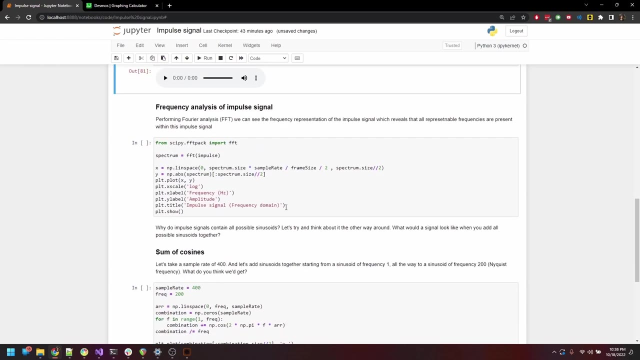 to 44.1 kHz. Well, this is what it sounds like: Unimpressive, obviously. What did you expect? It sounds like a click or a glitch. Now for the interesting part, If we take this impulse signal and subject it to Fourier analysis, 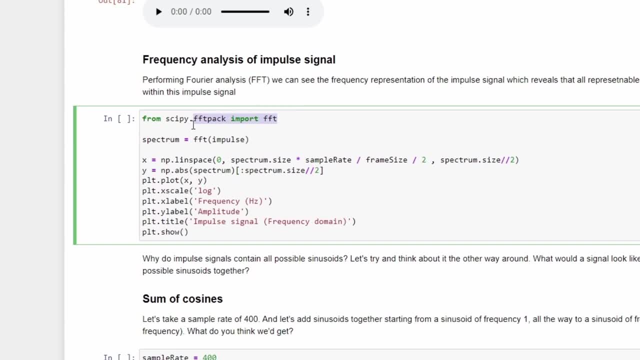 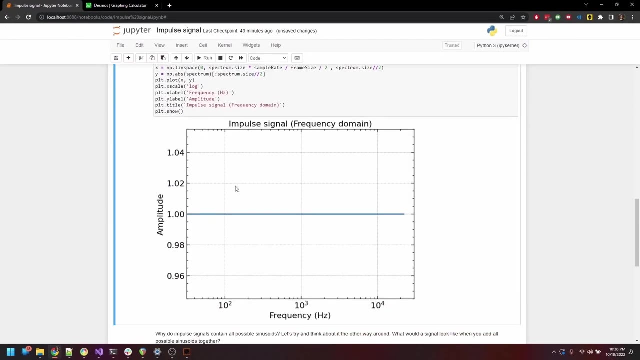 or fast Fourier transforms or the FFT algorithm. we can then get the frequency domain analysis of the signal. The output of the FFT operation is a complex signal, and if we extract the real part of this signal and then plot it on a frequency domain graph, we get this: 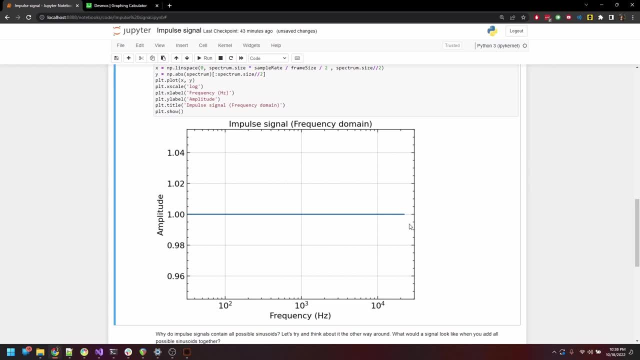 A straight line of magnitude 1.. This indicates that all the frequencies have a magnitude of 1. And hence all of the frequencies of equal magnitude are present in this line. Quite wild. if you ask me, We can use a more traditional spectrum analyzer to confirm this fact as well. 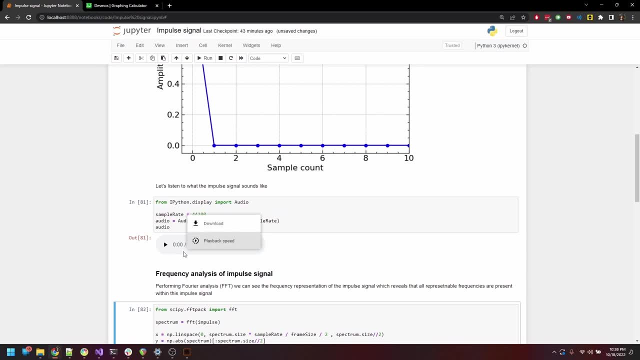 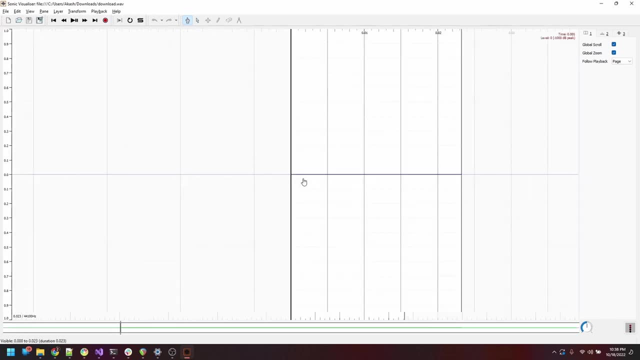 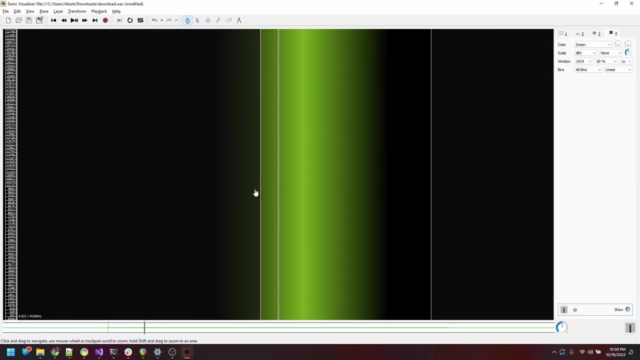 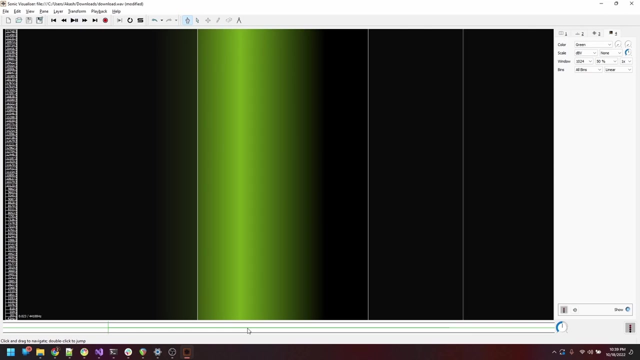 We heard what the impulse sounded like. Let's just write this out into a wave file and I'll import it into a sonic visualizer and open up the spectrogram And we can see again that all frequencies are present. But why? We see from the plots that an impulse signal contains sinusoids of every frequency. 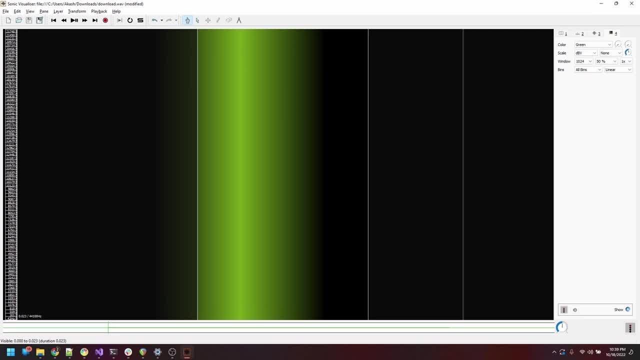 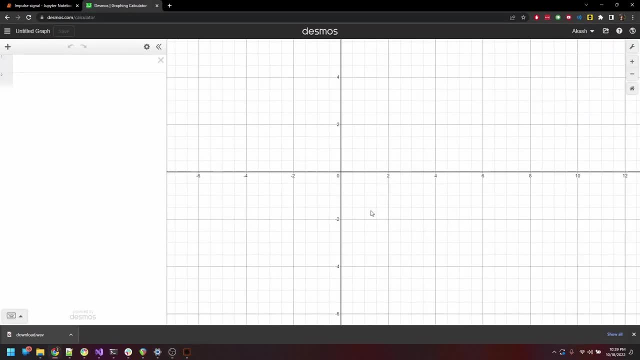 There's no denying that. But how can we build our intuition towards this fact? Here's a demonstration that might help. I'll head over to the Desmos graphing calculator And over here let's plot a sinusoid Y equal to cos. 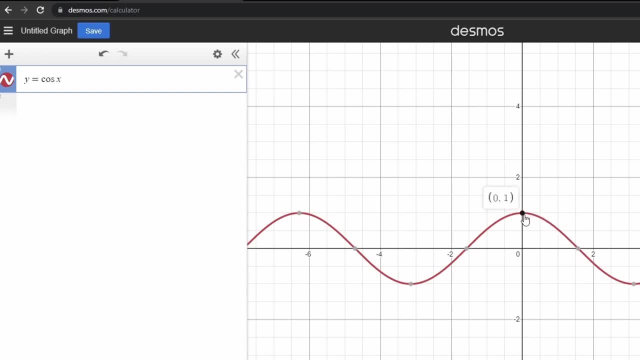 The reason why I'm using the cosine function here is because its peak falls at x equal to 0. This is a sinusoid with a frequency of 1 unit, let's say Now: the idea here is to add sinusoids of several different frequencies together. 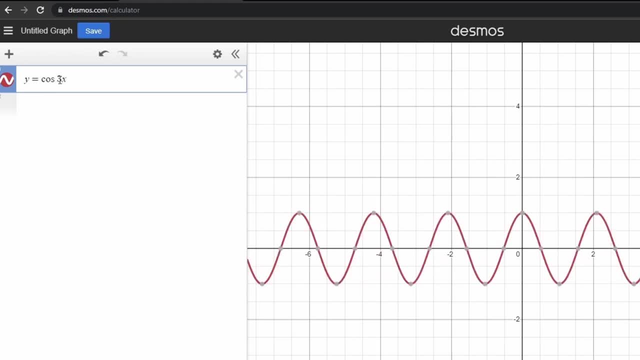 So this is a sinusoid with a frequency of 2 units and 3, and 4, and 5, and so on. We can see that for all of these sinusoids the peak coincides at x equal to 0. 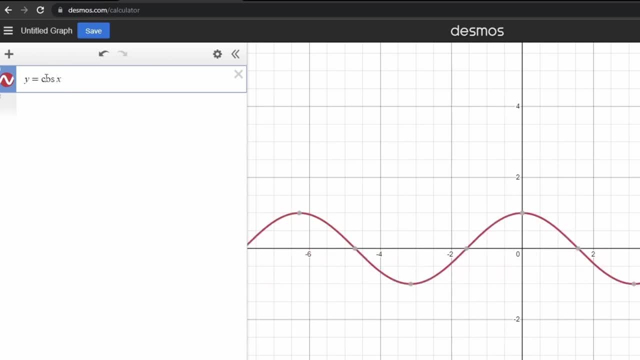 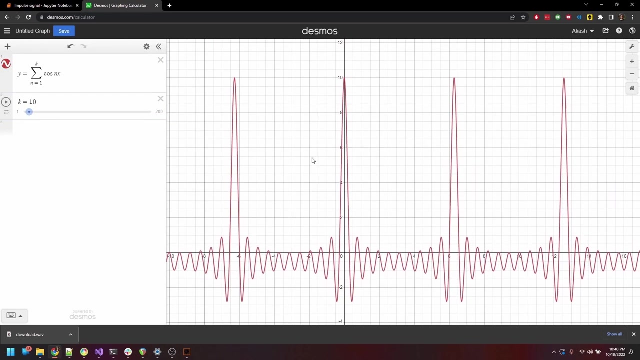 So if we add all of them together, the peaks constructively interfere. Let's write a simple summation of n values, where n goes from a value of 1 frequency unit to k frequency units, which is then controlled by a slider. As I increase k, we can see that the resulting plot has a local maximum at x equal to 0. 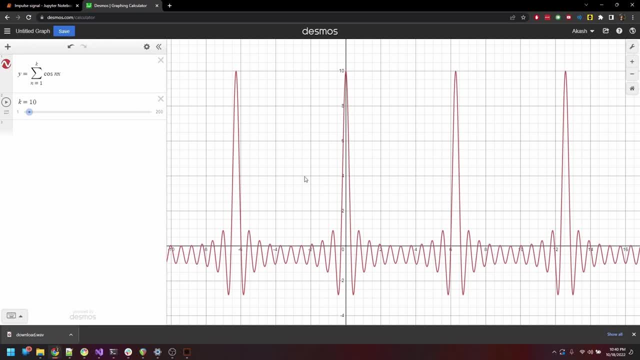 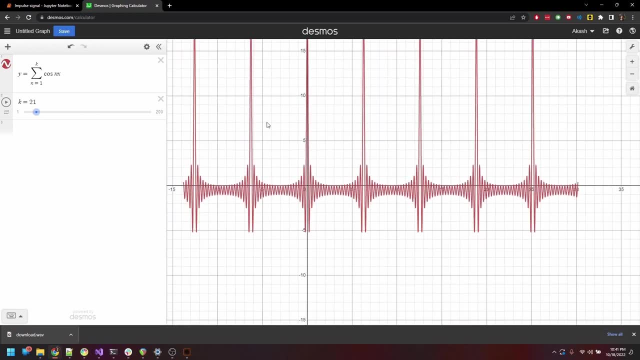 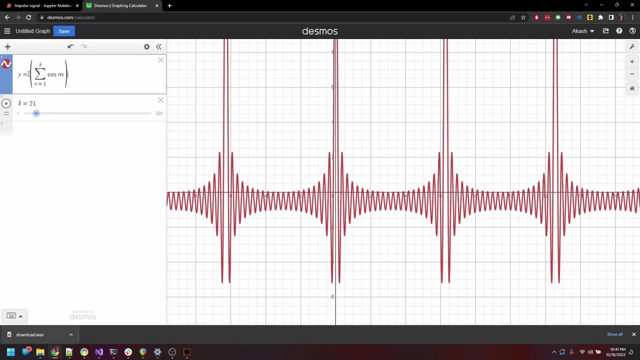 It has the same At several different places as well, but let's just focus on x equal to 0.. Since this plot will grow quite large, I'll normalize the values between negative 1 and 1, by just dividing the whole term with k. 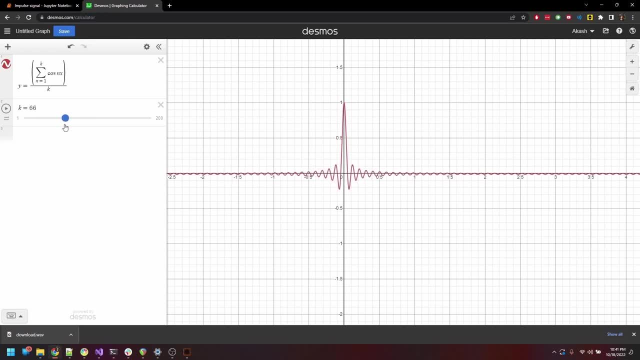 And now, as we increase k, which increases the number of sinusoids being summed, with the maximum localized value constrained to a narrower region, This is now at k equal to 200, which means that 200 sinusoids of increasing frequencies are being summed. 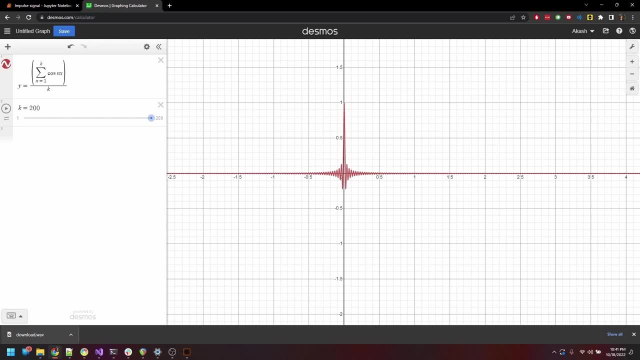 But, as you can imagine, if you keep increasing the number of sinusoids being added further, as this number tends towards infinity, the plot tends to become a unit impulse. But we are in the digital domain after all, so sinusoids with an infinite frequency is. 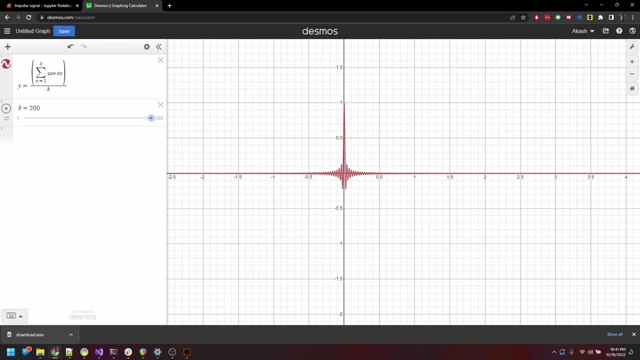 not something that we can achieve. We are governed by the Nyquist-Shannon sampling theorem. So if we were to take the sampling rate of k equal to 0, we would be able to calculate k equal to 0. But if we were to take the sampling rate of, let's say, 400 Hz, we can only represent. 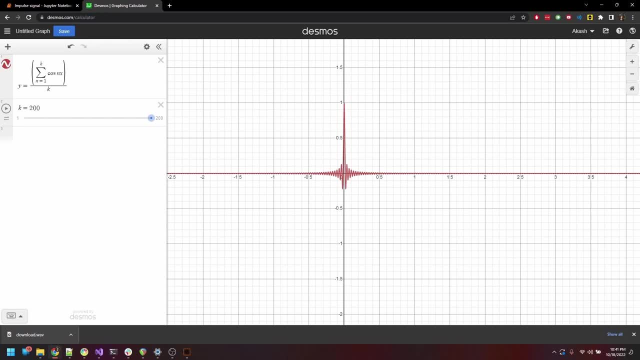 frequencies up to the Nyquist limit, which is 200 Hz. If we go by the Desmos calculator, we are already at the combination of sinusoids of up to 200 frequency units, But there isn't a single point, like we saw in the impulse signal. 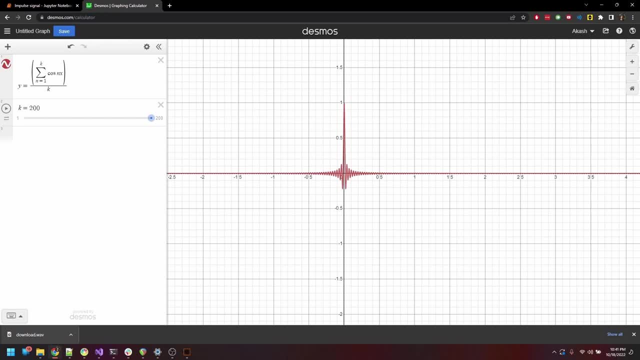 Obviously, we are looking at this from the lens of a continuous time system. If we were to take this same signal and discretize it at the sampling rate of 400 Hz, we'd get a single point, since at that sampling rate only one sample gets quantized to 1, and the 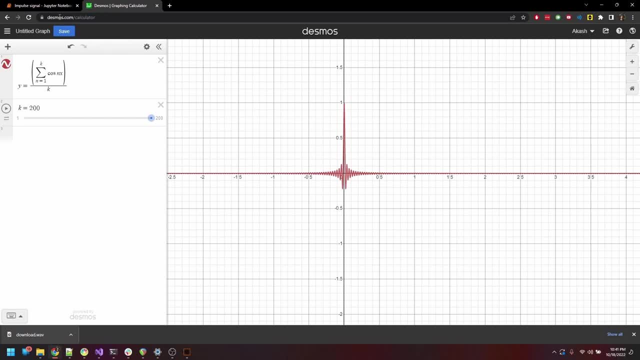 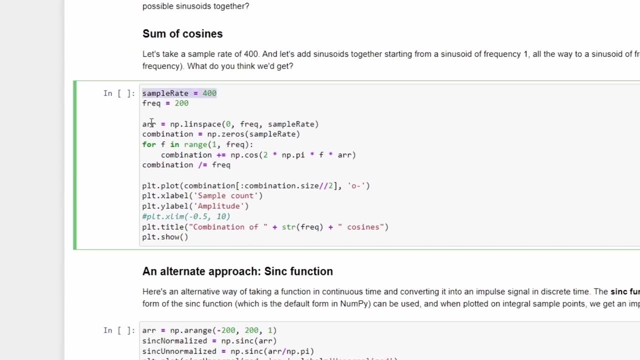 rest of the samples are quantized to 0.. I can quickly demonstrate this by adding an arbitrary number of sinusoids in the Python script. If we take a sampling rate of 400, and any frequency less than 200, and plot only a period, 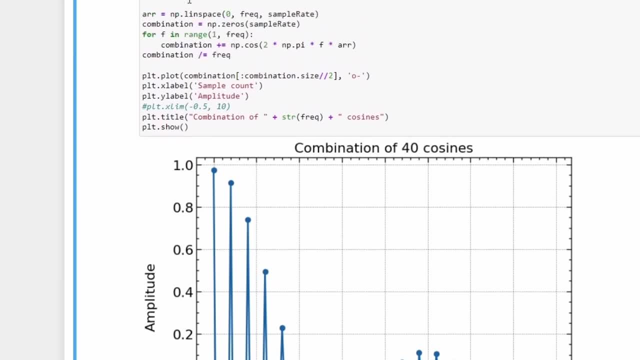 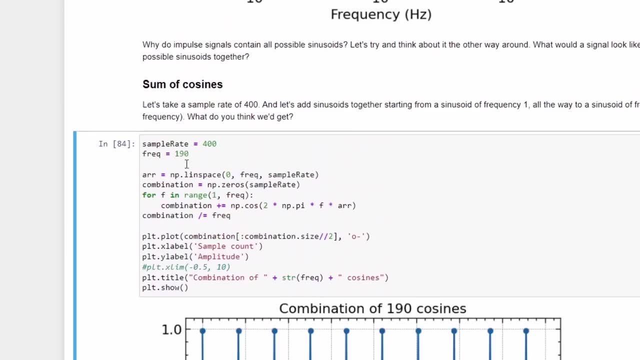 of the waveform. we can see that in the discrete form it's an arbitrary waveform. But as we approach a frequency closer to 400, we can see that the sampling rate is equal to the sampling rate of 400.. If we approach a frequency closer to the Nyquist, closer to 200, we get a signal which closely 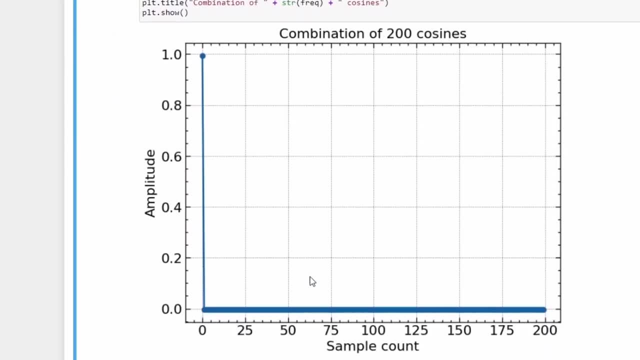 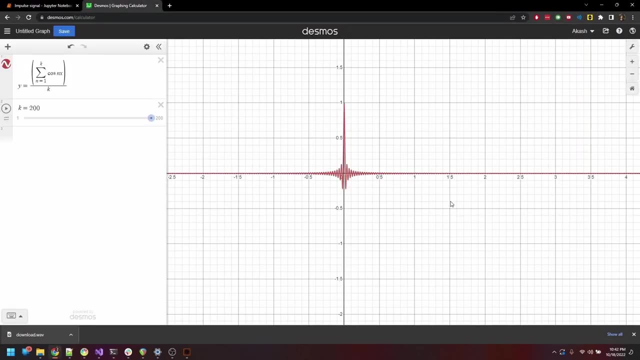 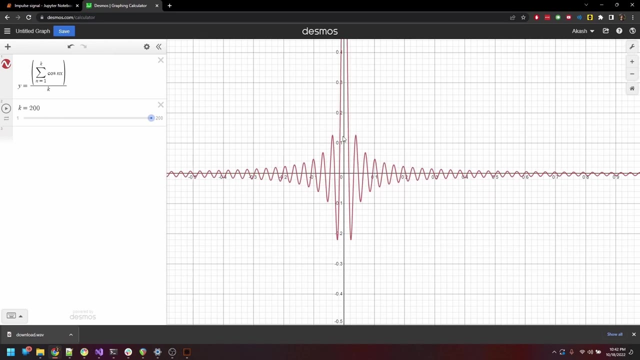 resembles an impulse And at exactly 200, we get exactly that: we get the impulse signal. So what we see here is a continuous time equivalent of a discrete impulse signal. And this continuous signal has special significance and it's called the sinc function or the 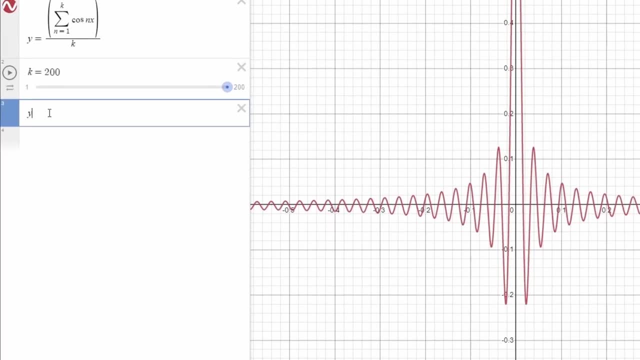 sine cardinal function. The function definition of the sinc function is basically sin. So what does that mean? It means the sum of x over x And the sine of the sine of x is the sine of x over x, ie the sine of kx over kx. 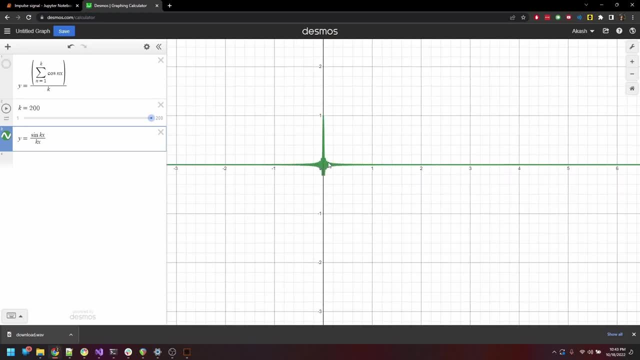 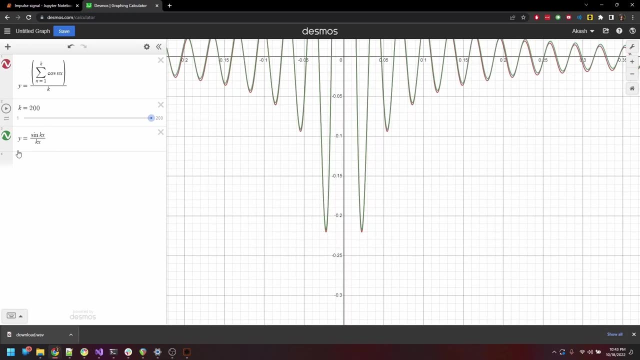 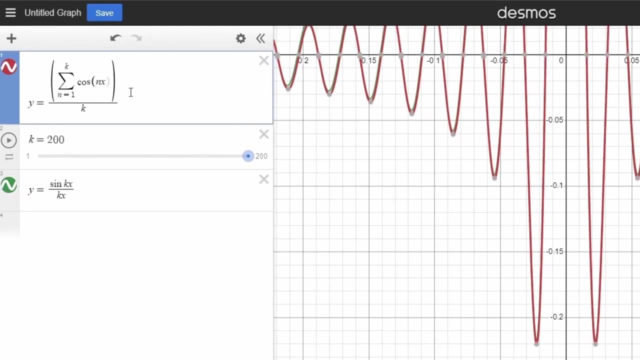 The sine of the sine of kx over kx is essentially the sine of kx, ie the sine of kx over kx, And it's quite similar to the summed cosines. In fact, if I change this term slightly, the two signals are equivalent. 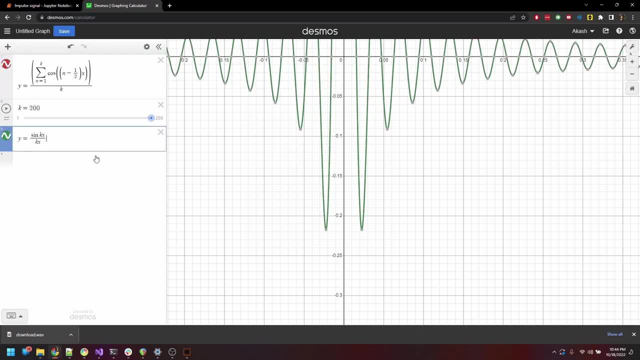 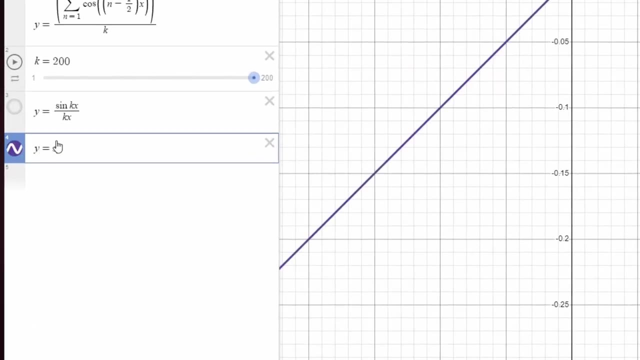 The sinc function is quite useful in signal processing for a variety of reasons, but in this video we'll see how a sinc function in continuous time is actually just the impulse signal in discrete time. There are two general variants to the sinc function: the unnormalized form, which is 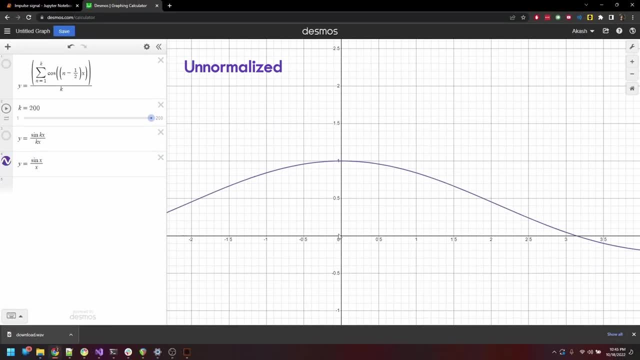 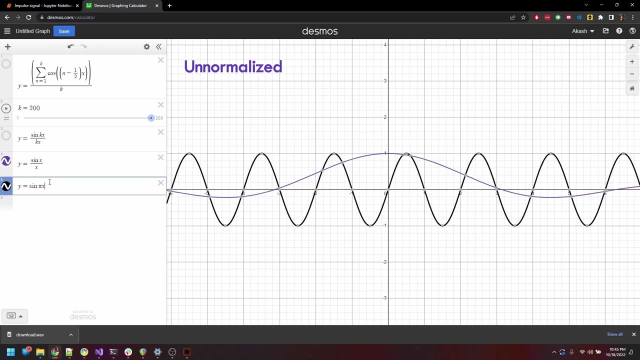 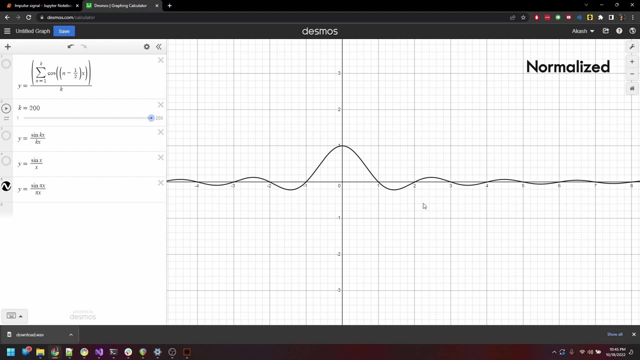 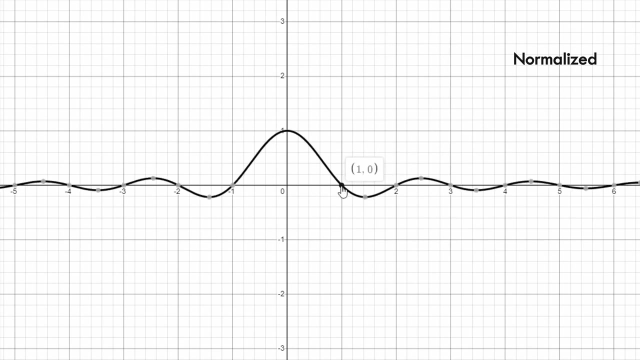 sin over x and the normalized form, which is sin over pi x. The normalized form is the most useful form of the sinc function in signal processing and we can actually see why: At x equal to 1 on the number line, the sinc function equates to 0. 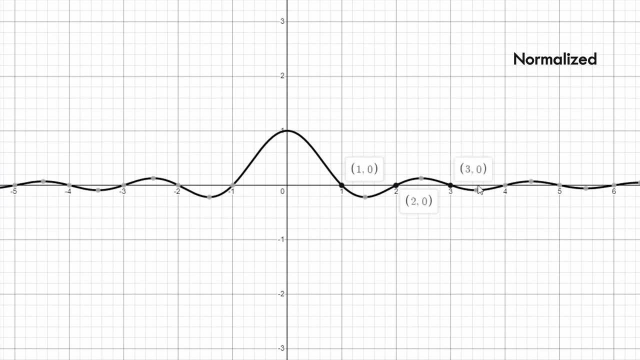 It's 0 at x equal to 2, and at x equal to 3, and x equal to 4.. It's 0 as well. Going over to the negative axis, it's 0 at negative 1,, negative 2, and so on. 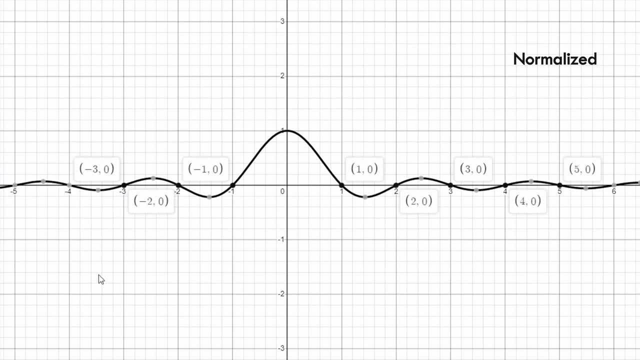 So at every integral point on the number line except for x, there's a sin over pi x, At x equal to 0, the value of the normalized sinc function is 0. And we can imagine what this means in discrete time. 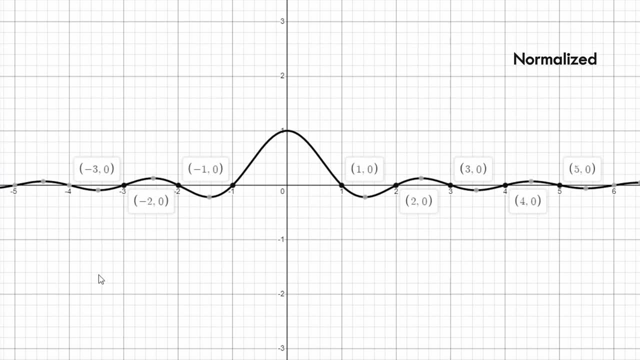 In discrete time. we sample this signal and capture values at discrete intervals like 1,, 2,, 3, and so on, and discard the values in between. So if we discretize this normalized sinc function, we get an impulse signal. 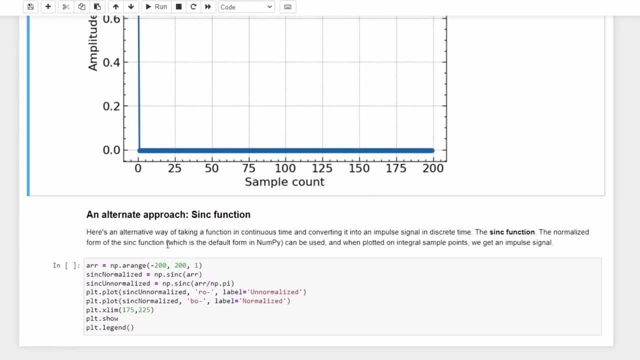 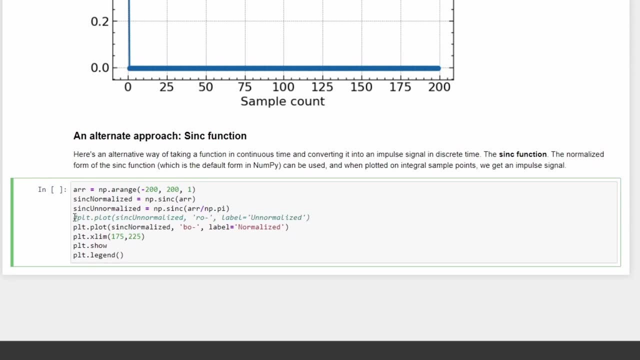 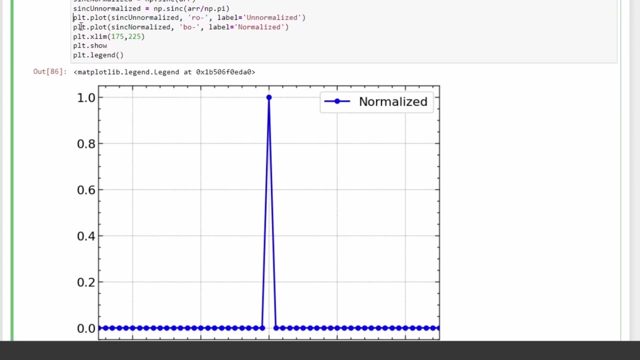 In the script. we previously got an impulse signal by summing up all the frequencies up here, But now all we need is a single normalized sinc function and we get an impulse signal. We can see the form that the sinc function would take if it was un-normalized, and it